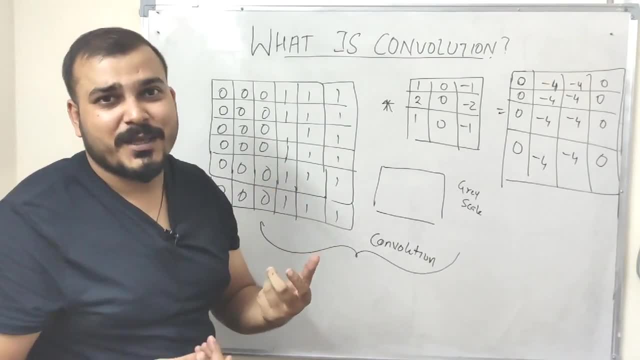 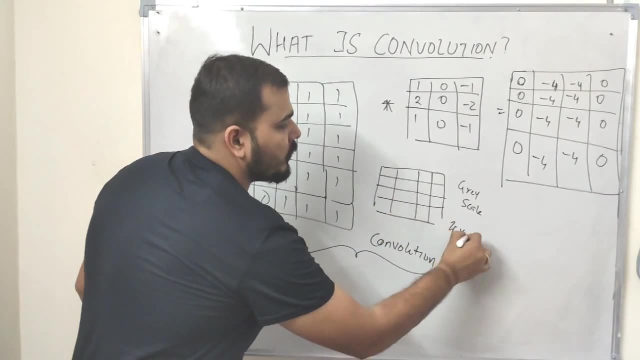 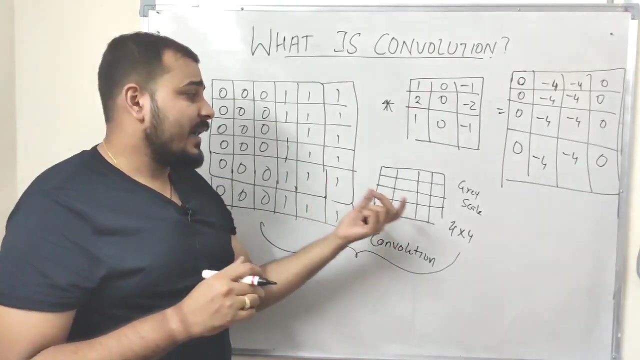 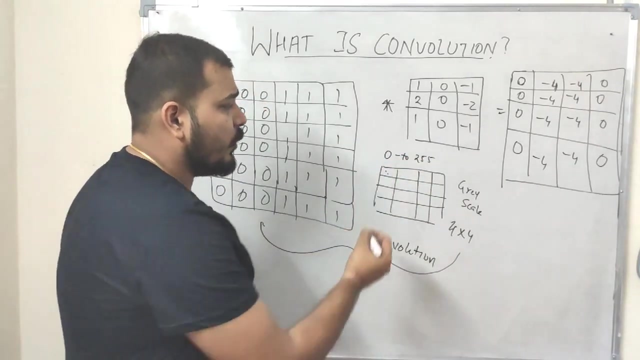 It may be 200 pixels into 200 pixels, It may be 6 cross 6 pixels. So let me just consider this particular example. Suppose I consider this is my 4 cross 4 pixels, So this is my 4 cross 4 pixels. And when I say grayscale, that basically means that this particular image has black and white kind of stuff. Okay, black and white colors. So most of the values of this pixels ranges between 0 to 255.. So every value in this particular region, it may be 255, it may be 128, it may be 24, it may be 255., 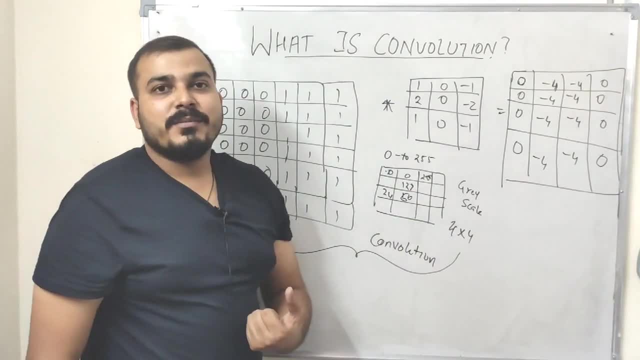 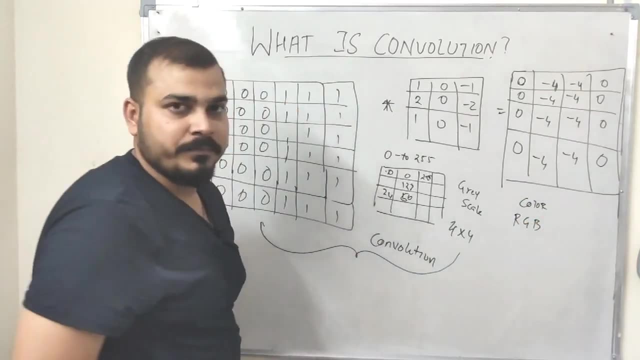 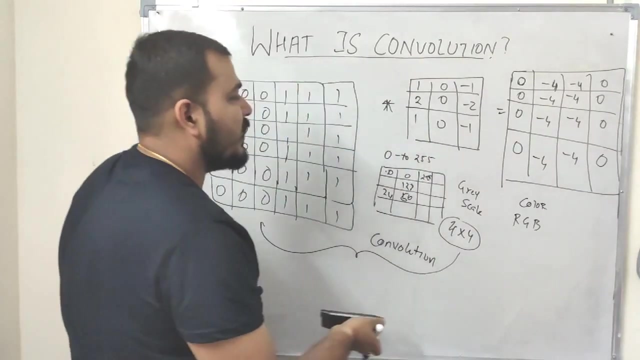 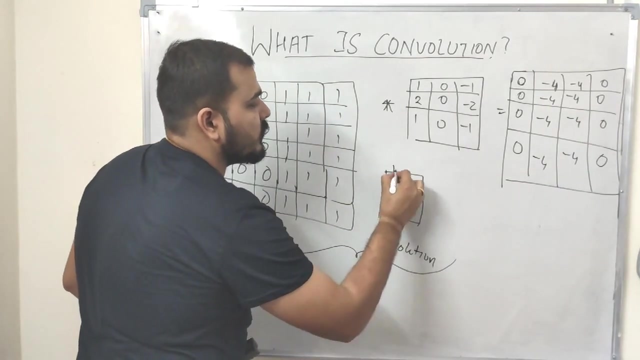 It may be 50. And based on that, that particular image is basically displayed. Similarly, there are some colored images also. Now, colored images is basically with the scale of RGB. So if I want to specify this image, I'll write 4 cross, 4 pixels. But in case of RGB, our RGB image will look something like this: Suppose I have my R channel, Okay, this will be my G channel, this will be my B channel. When this all is combined, we basically get 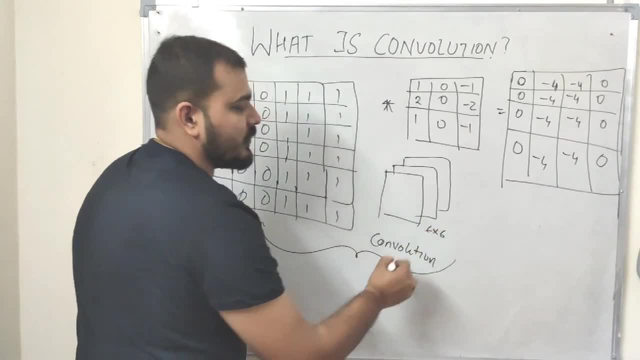 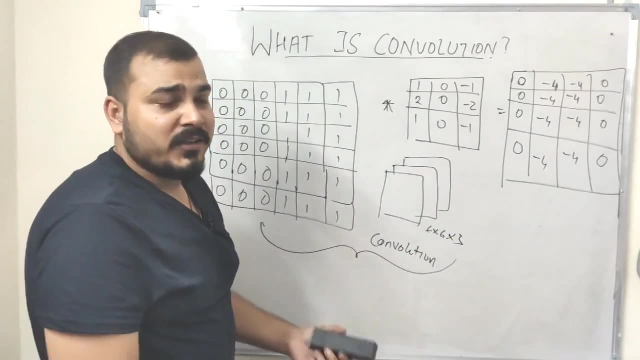 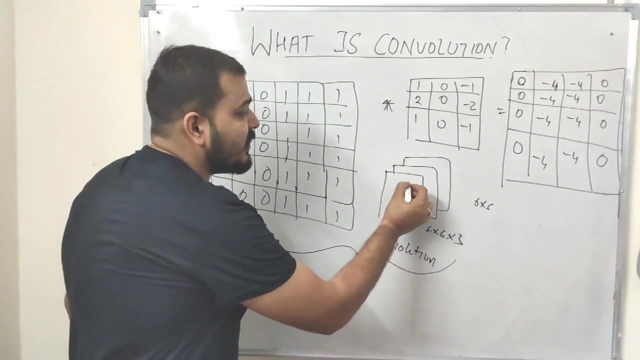 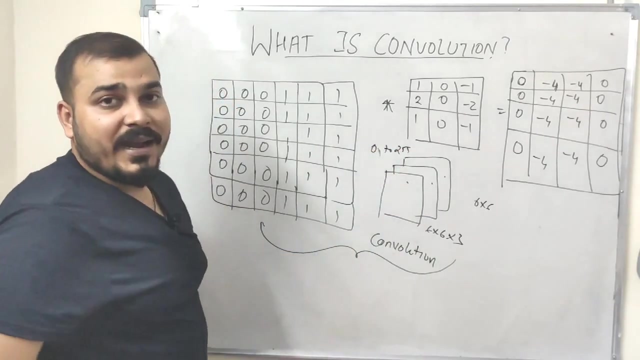 a colored image And again, this can be any number of pixels: C cross 6.. But here I have three channels. it is basically specified as 6 cross, 6 cross, 3 channels. Okay, in the case of grayscale, I'll just write 6 cross 6.. In case of this it will, I'll try to specify this third channel And, as I mentioned that this, each and every color channel, also, the pixels will be between 0 to 255.. Okay, And again, remember guys, we can also reduce or normalize this pixels also. 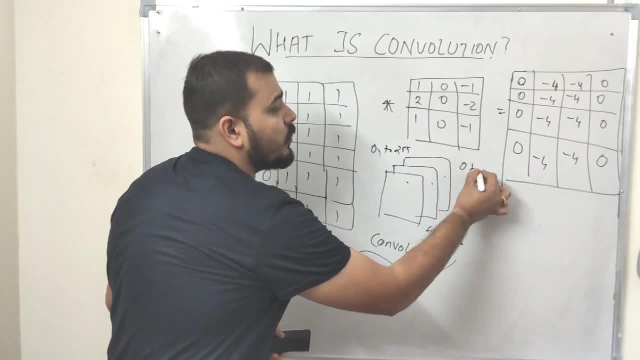 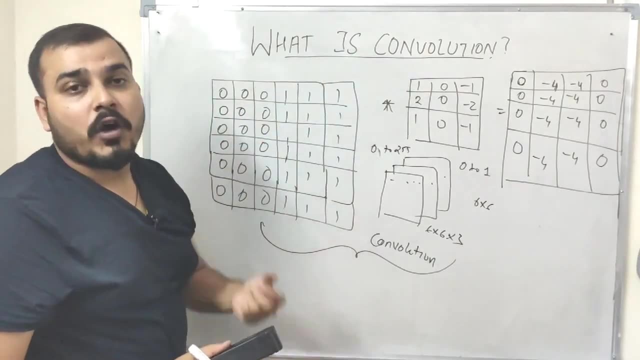 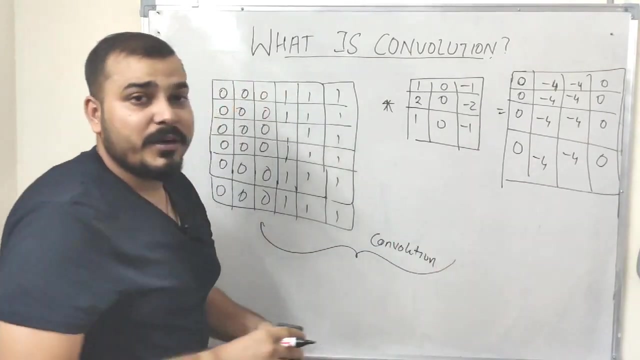 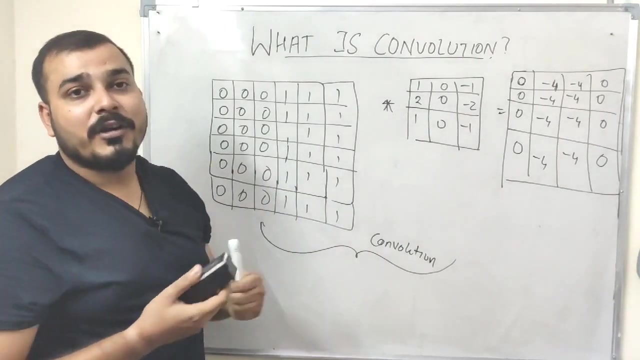 If I use min max scalar, this will get reduced between 0 to 1.. You know each and every pixel values will be getting 0 to 1.. And that same example I'll be showing you here and what exactly convolution will try to understand also. So this was some basic information about this images. I probably think you may have gone through this in your computer graphics. You know there was a subject in computer graphics related in engineering. I hope you may have understood about that basic stuff. Now let us just go and understand. This is the first. 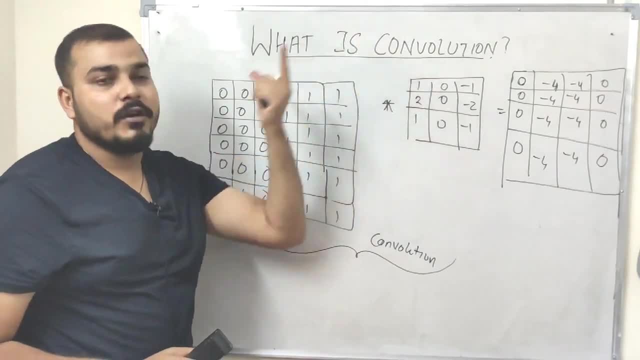 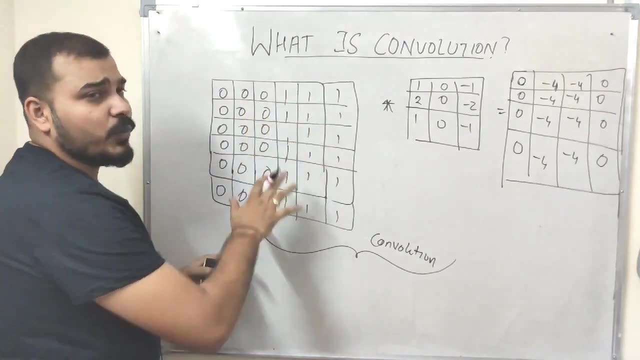 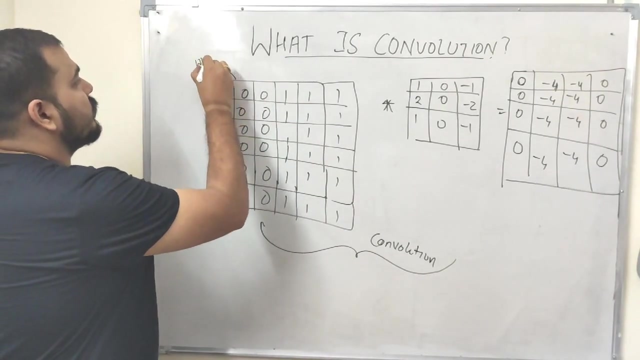 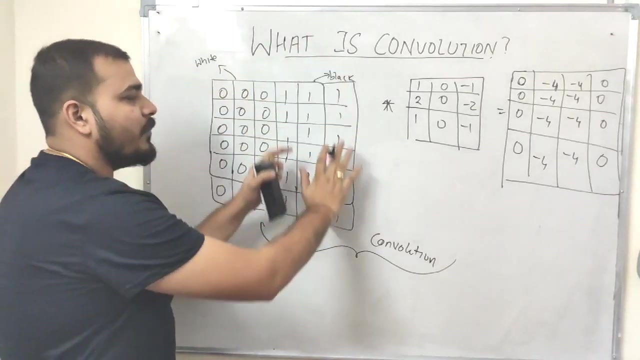 component of the first basic step of a convolution neural network, which is called as convolution. Now let us consider this particular image. Now, this image: I have basically scaled down between 0 to 1.. And suppose I have just zeros and ones values. This basically indicates that zero is basically my white, white color. suppose one is basically my black color. Okay, Now, here you'll be seeing. this will be completely white, this will be completely black. Now remember, guys, in my previous video I told you about the human. 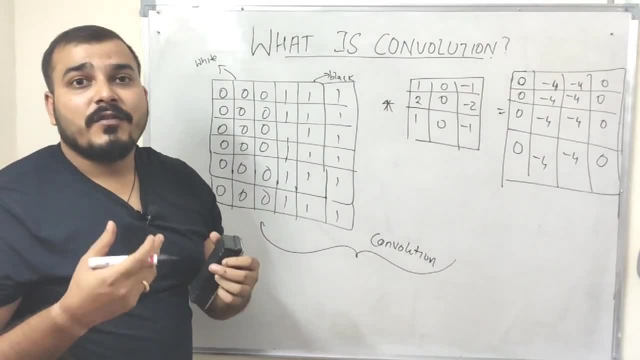 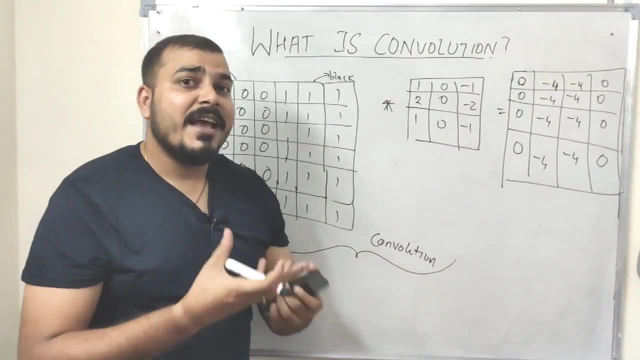 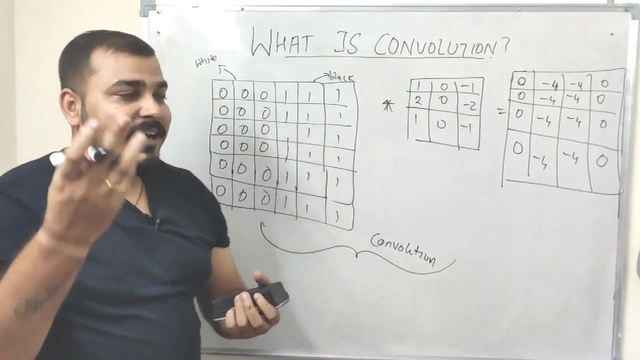 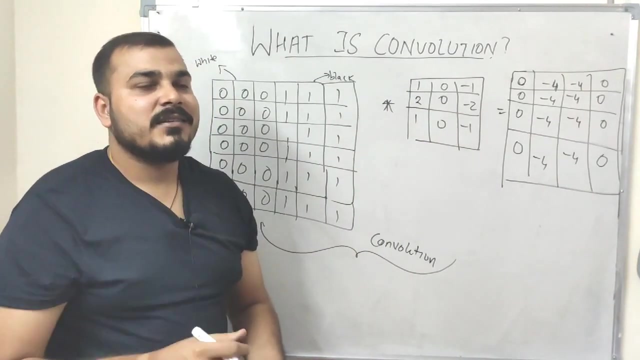 brain right, The main part, which is basically responsible for seeing the images. I told you about various layers like V1, V2, V3, V4, V5, V6. I told you that each and every layer was very much responsible for finding information from the images And I told you that that were acting like filters. Now, this is the filter I what I was talking about. Suppose, consider that after I pass that particular image, V1 layer is responsible for finding the edges. That basically means V1 has this kind of filters. 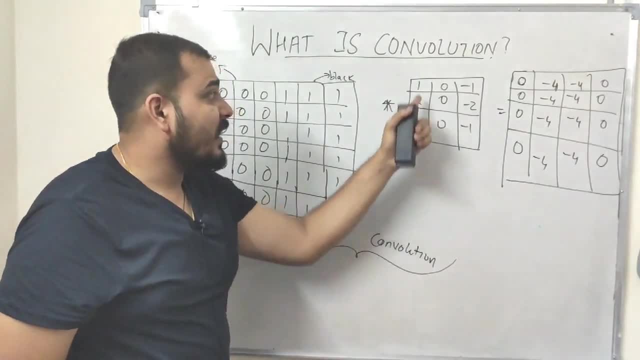 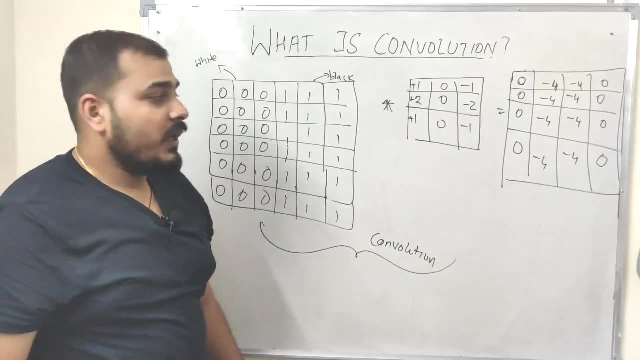 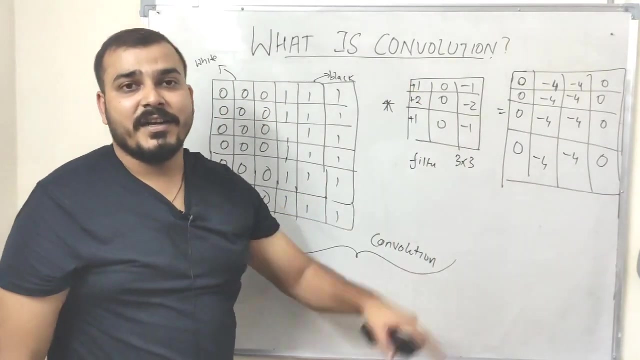 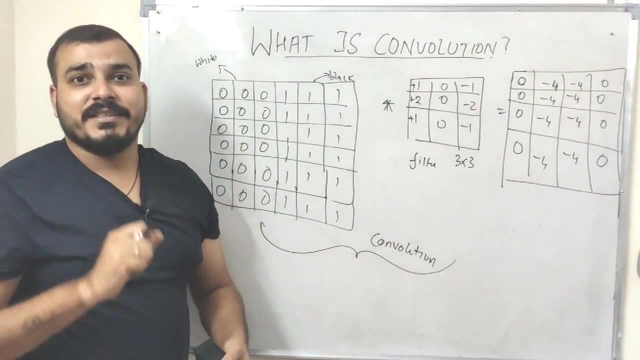 Okay, now this particular filter that you see, and I have specifically written like plus one plus two plus one, because this is something called as vertical edge filter. Okay, and we specify this as a filter. Okay, so this, this three cross, three matrix over here, is basically a vertical edge filter. That basically means that if I apply this filter on any images, it will be able to determine all the vertical edges. Now, in this case, you have vertical edges over here. So this is your white color, this is your black color. 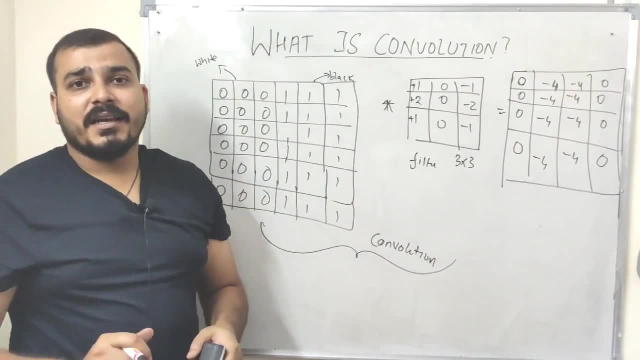 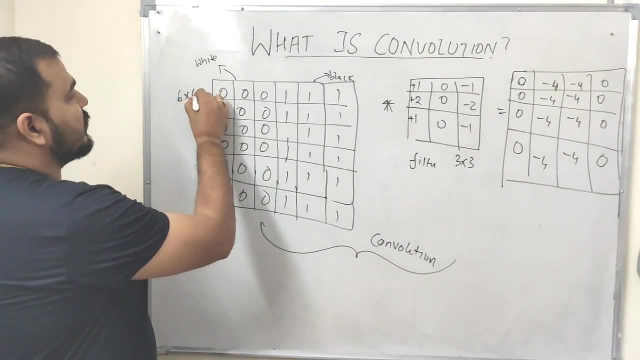 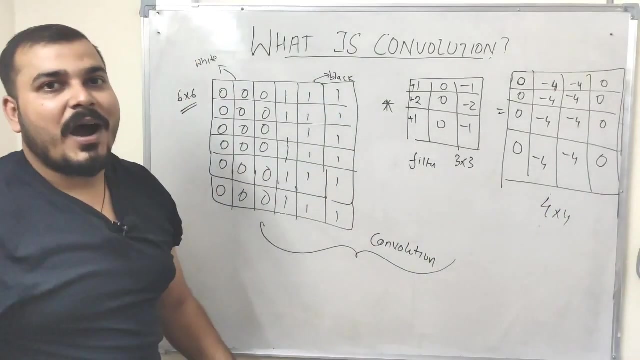 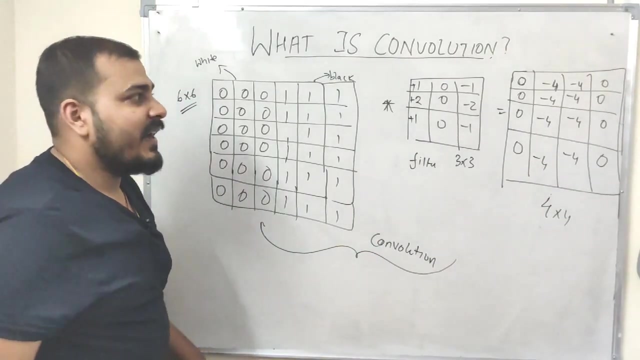 So here in between, you basically have a vertical edge. Now let us see how this convolution operation actually works. Now remember, guys, this image is basically six or six pixel. When I apply a filter, three cross three, I'm getting the output as four cross four. I'm going to show you how we are actually getting this output as four cross four also. So let us begin. In order to apply convolution, all we have to do is that place this filter on top of this particular image. So here you have three cross three. So let us begin. 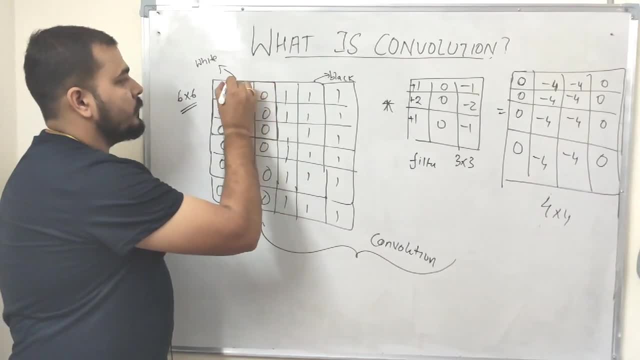 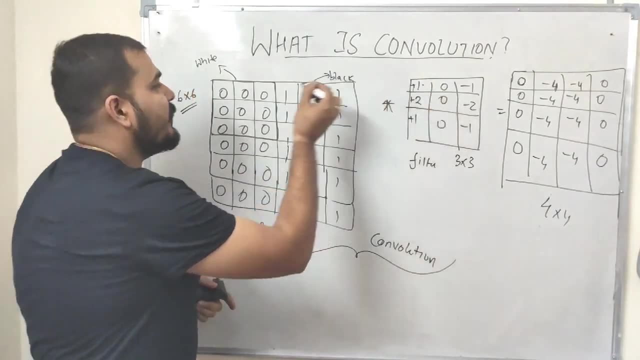 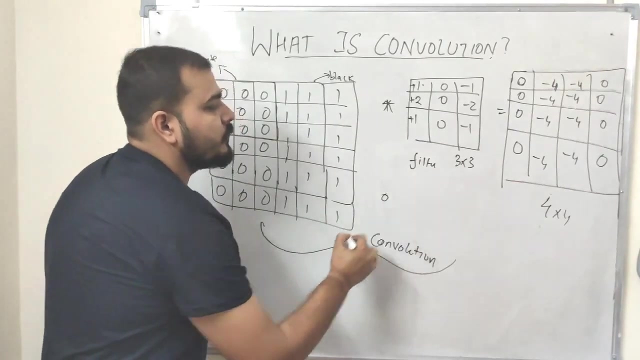 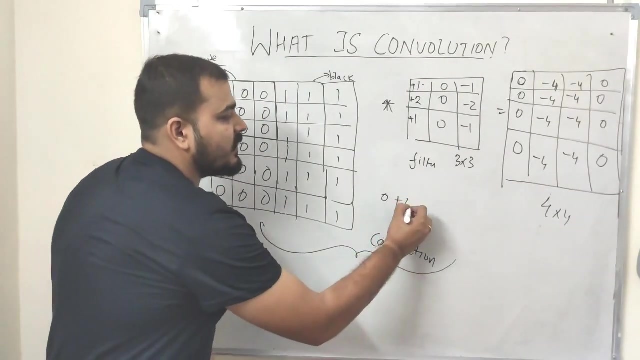 Let us take this three cross three initially. Okay, so when we take this three cross three now you see over here, all you have to do is that multiply this term with respect to that particular cell. So in the first case, you see that plus one will be multiplied with zero. So I will get zero. then I will add the next value. this zero will get multiplied with the next zero. Okay, again, I'll be getting zero. Now, similarly, minus one will get multiplied to this zero. and we have to also do the submission. 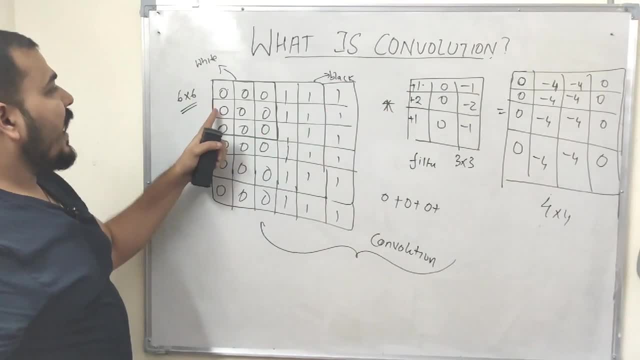 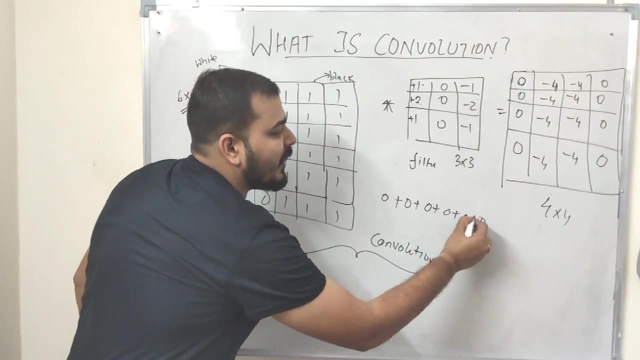 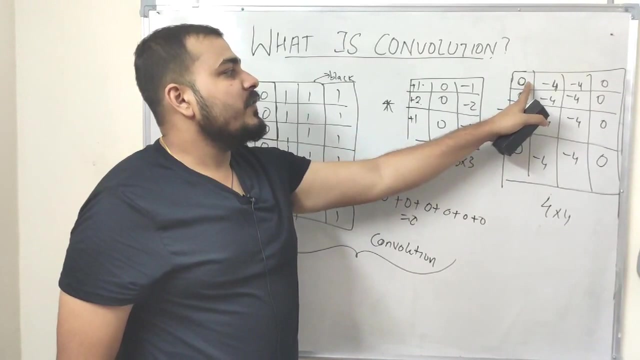 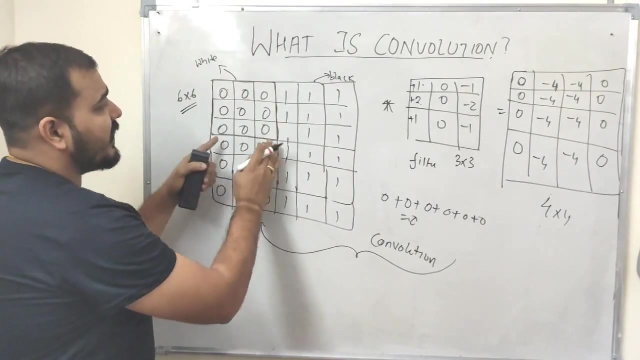 And I'll get this as zero. then I'll go to my next row And this zero will get multiplied with this, this will get multiplied with this, this will get multiplied with this, And, similarly, you'll be seeing that everything will be coming as zero. So, when you see all this value, once you calculate the sum, it will be zero. this zero, you have to replace it in your first cell as your output. Now, once you do that, the next thing is that now this is my three cross, three right. Next, I will be doing a stride jump of one. Okay, so I'm going to do a stride jump of one. 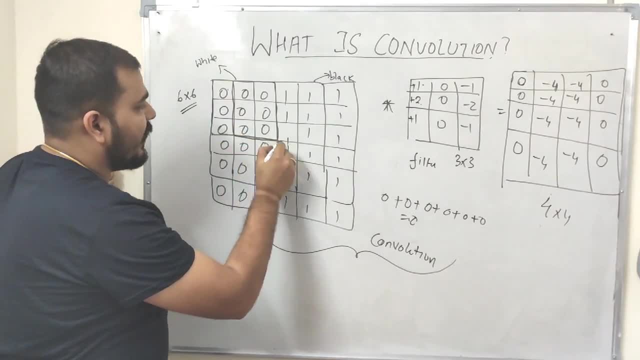 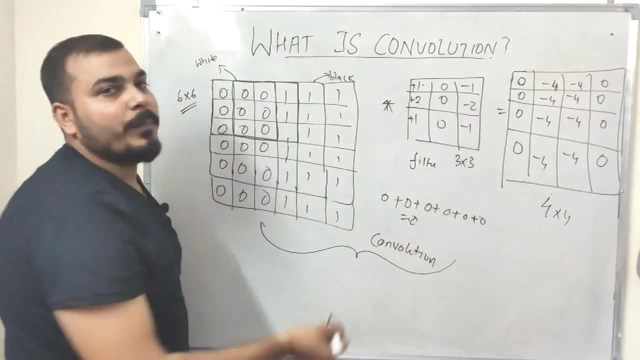 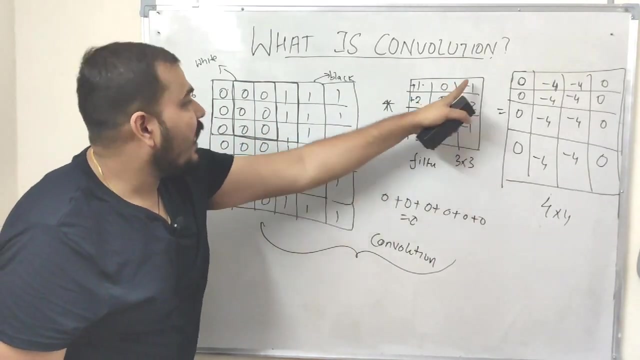 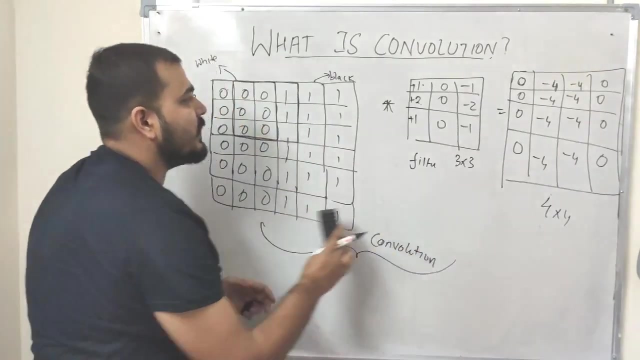 A stride jump of one basically means that I will go and select my next cell by jumping one to the right, like this: we'll just move one step forward And I'll go and apply the same operation. Now, here you see that these all are zeros, right? So I will basically be getting initially, for all these values, zeros, but for the last layer I have 1111.. So, in short, this will get added. So this, my first value will give it added like this: Let us see: this value will get multiplied to this, So it will be zero plus, zero plus when this value is. 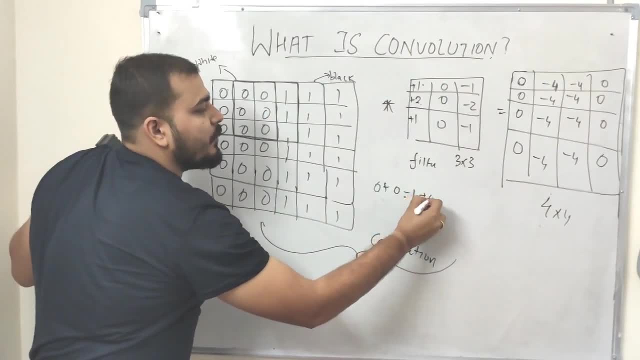 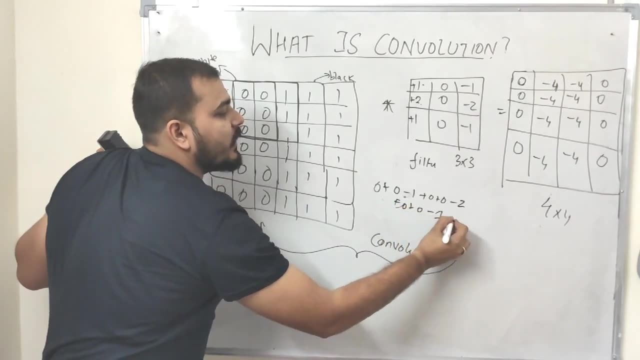 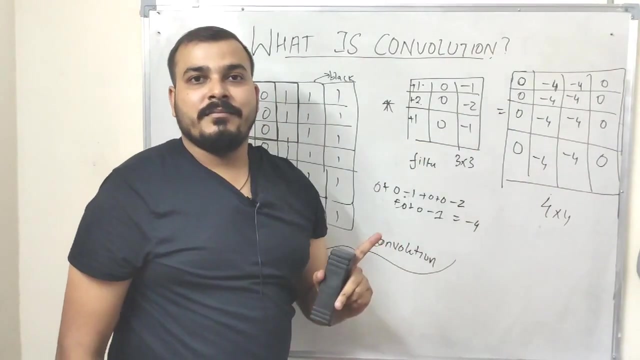 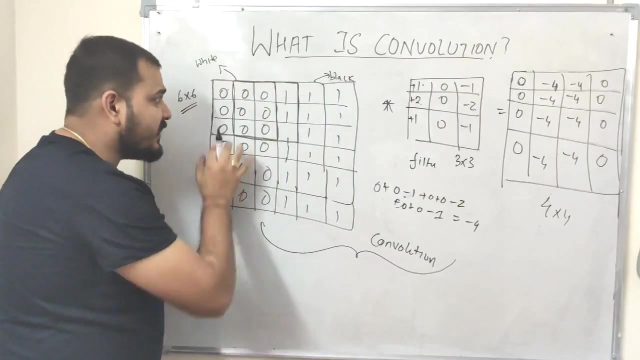 getting multiplied to this, this will become minus one. Similarly, plus zero plus zero. this, when it is this getting multiplied to this, will become minus two plus zero, plus zero. then it will be minus one. So the total output that I will be getting is minus four And that thing. I'm trying to replace it over here, And I'll do it for each and every field. I'll make the stride jump one by one, But once it comes over here, we have to come one step down. That basically means you have to start it from here again Every time we have to. 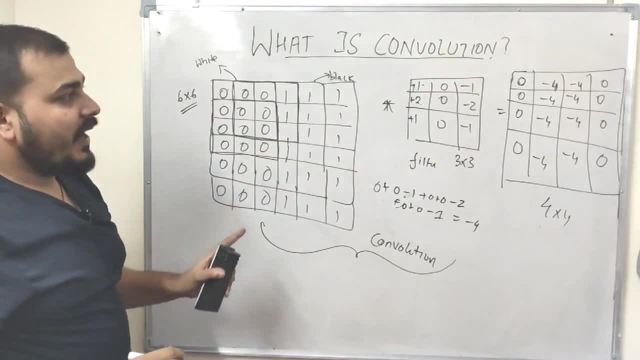 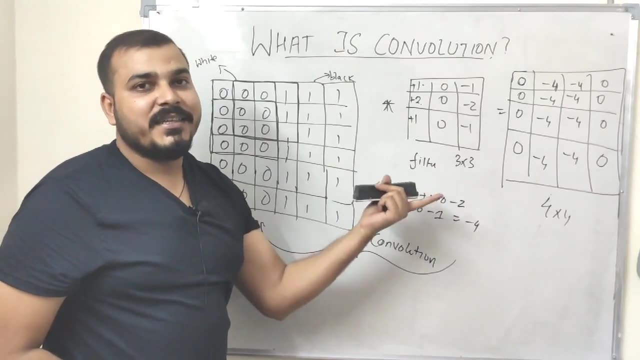 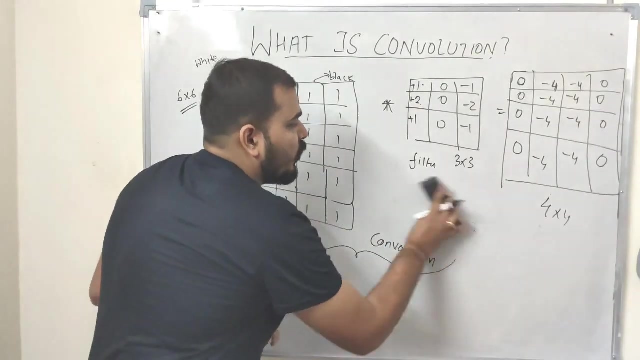 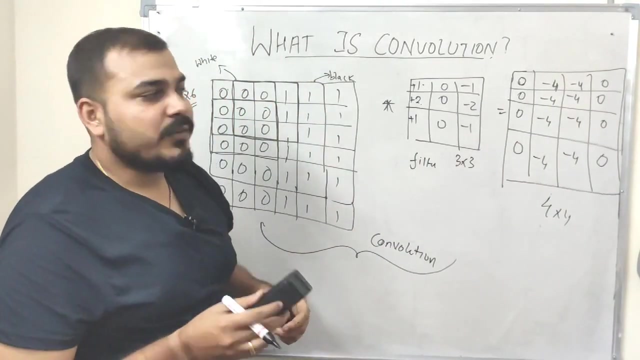 do one step down after we complete the end of the image, And similarly, we'll be filling all these details. Now, this is a filter. I told you this filter is basically a edge vertical edge detector. Now, based on the output, we'll try to understand what is exactly vertical edge detector. Okay, So what I'm going to do is that, after I get this particular output, I can again re transform this image by using min max scalar, min max scalar. what it does. over here you're trying to find out the min value. the min value is minus four, right? So 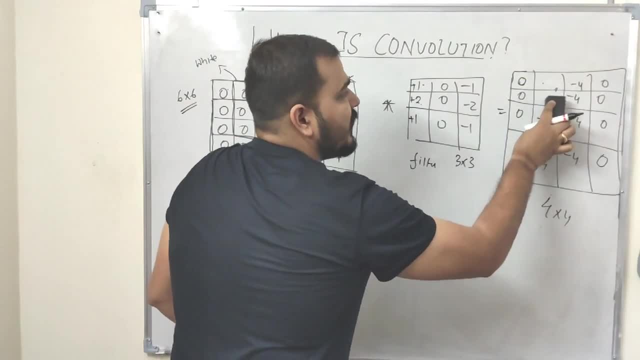 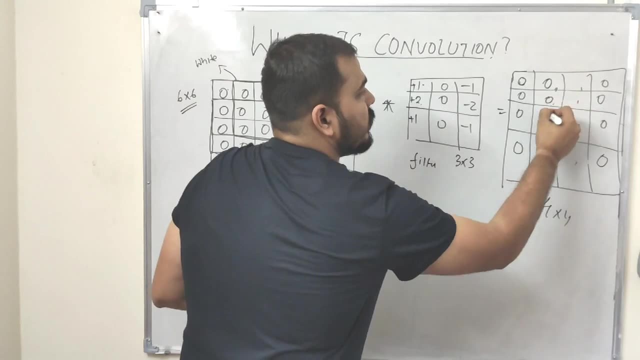 if I think to the value, what it does over here. So at this point my scale value, my min 150, finite yüzde and zero is the max value, So I can actually change all this min value to zero. See, I'll change all these min value to. 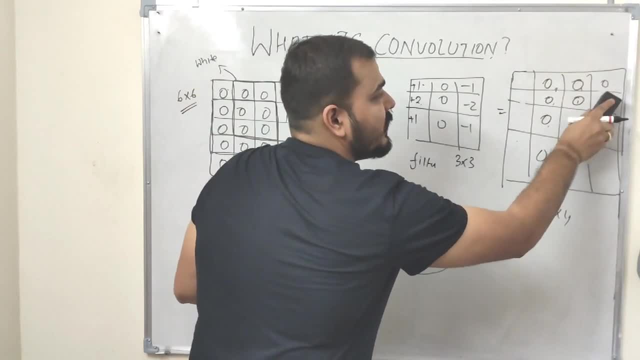 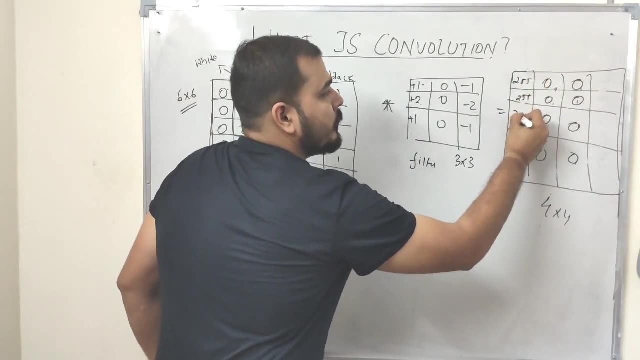 zero by applying min max scalar and this max value that I had a zero, I had convert this back into G 55, because the maximum pixels in an image is 255, right, Because of the min max scalar value I had applied earlier. So this will become 250. 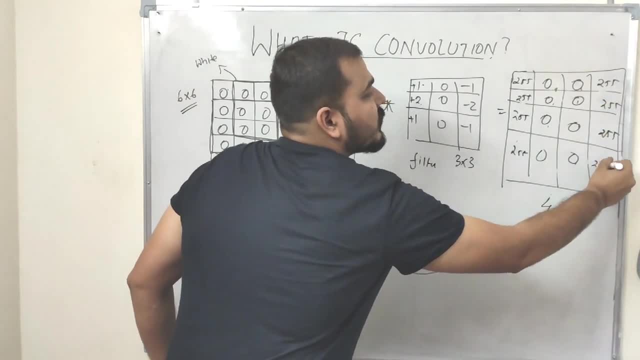 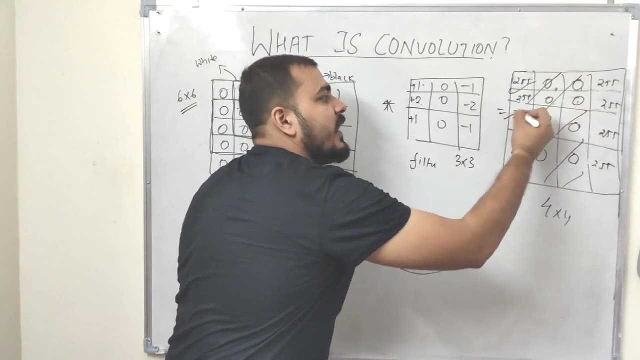 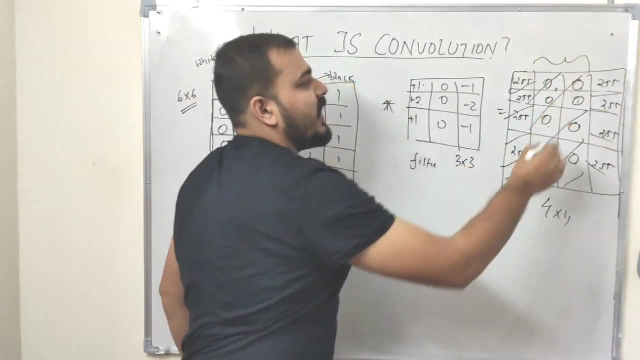 the pixels will get converted by applying the min max killer. now, what do you see from this image? the middle layer is basically a white side. this is completely a dark side, right? so this is your dark, this is your white, this is your white, and this white is specifically determining the details of 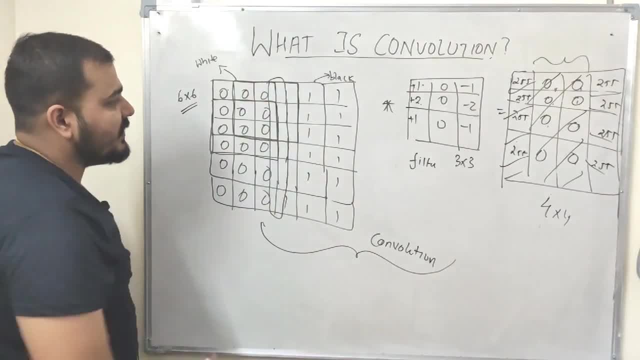 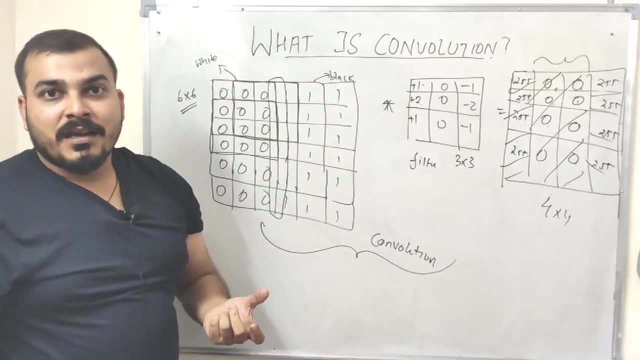 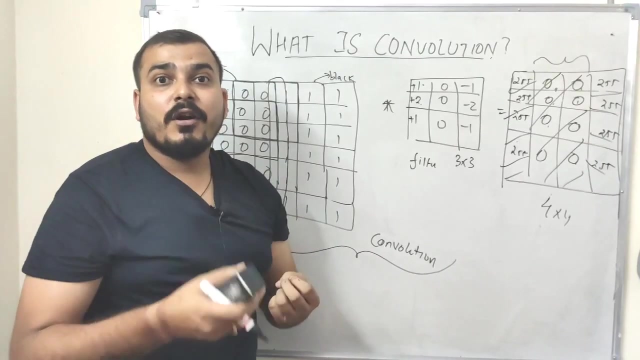 this edge of this edge, because I told you there is a edge between this white and black color, right? so this particular edge is basically determined by this particular filter. now, understand that this filter plays a very major role over here, because when we'll be having v1, v2, v3, v4 layers, at that time this v1 suppose- 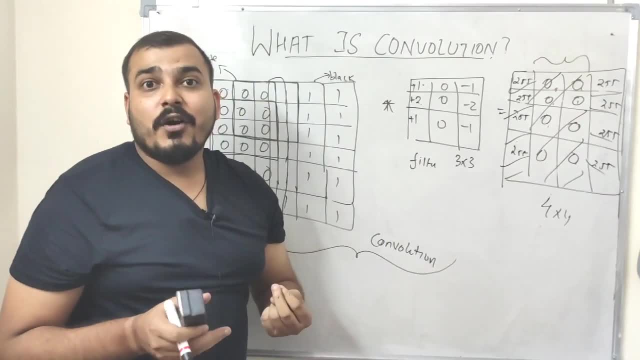 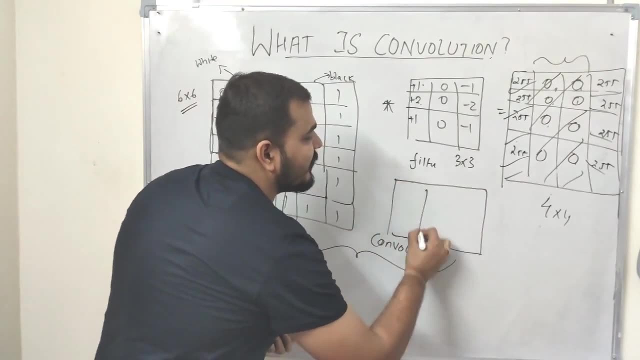 it is doing a vertical edge detector and suppose after that v1 also has the capability to doing for doing a horizontal edge detector. horizontal edge detector filter will look something like this: it is very simple common sense. again, if you want to find out about various filters, you can just do. 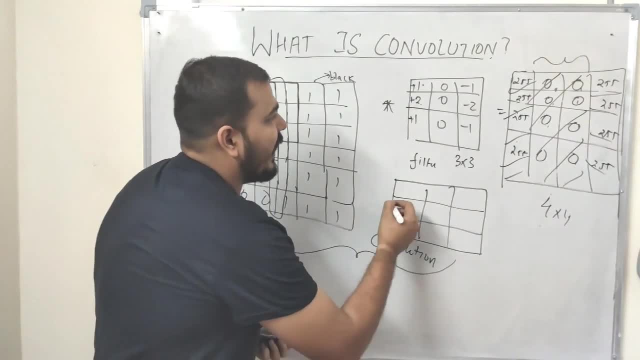 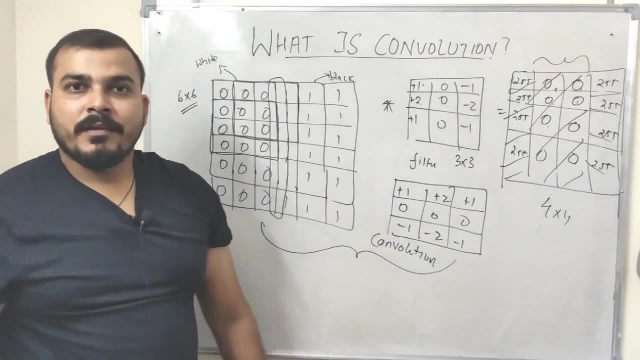 Wikipedia and you can just extract all the details so you'll be able to find it in this particular filter, and you can just extract all the details so you'll be able to find it- that your vertical edge detector will look something like this. okay, so this is the basic funda all together. okay, so like this. now for this image now. 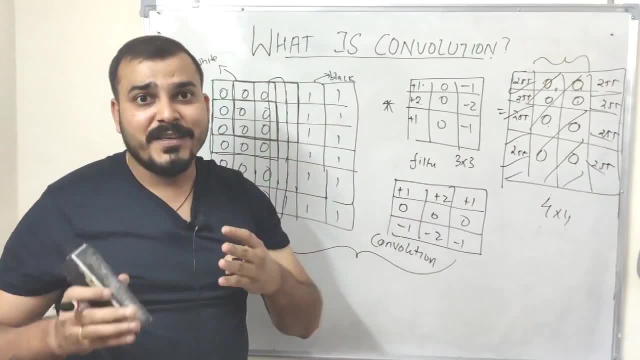 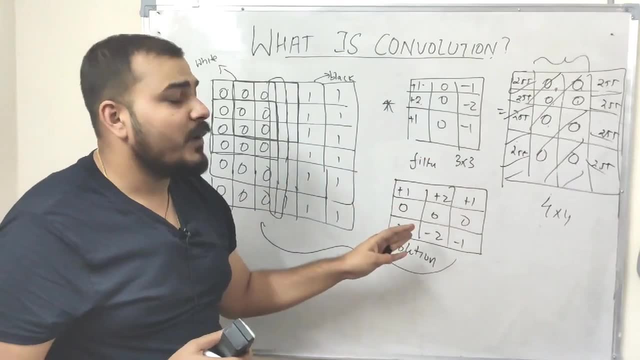 see guys in in our human reign. I told you where you have various layers, from v1 to v6, like this, v1 to v6. just understand that if I create multiple filters like this, one filter will be responsible for calculating the vertical edge. the other filter will be responsible for calculating the horizontal edge. the other 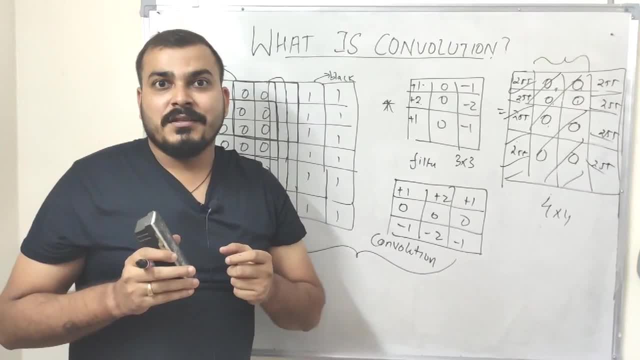 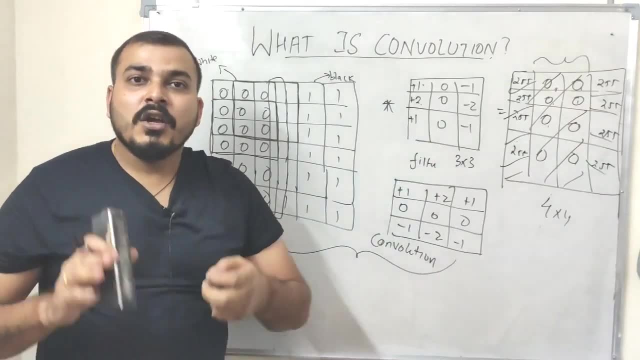 filter will basically be responsible for finding the edges of the face. So different, different, different filters are already there, present over there, and you'll be considering that. how can we design this? You don't have to worry about that When we are implementing with the help of Keras. 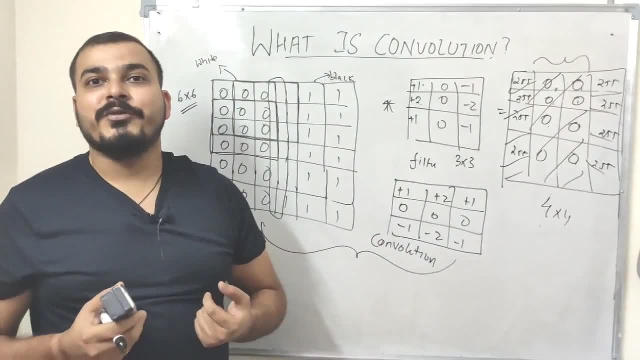 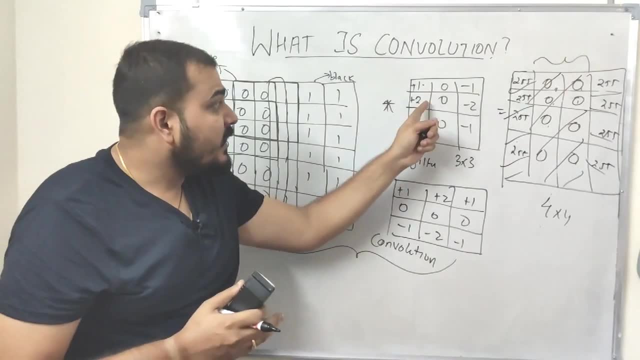 you just have to specify your filter size and how many number of filters you want to use. It will consider all the necessary filters and later on during the training for that particular filter, will be updating these values also, like how we updated the values for the weights. So with that, 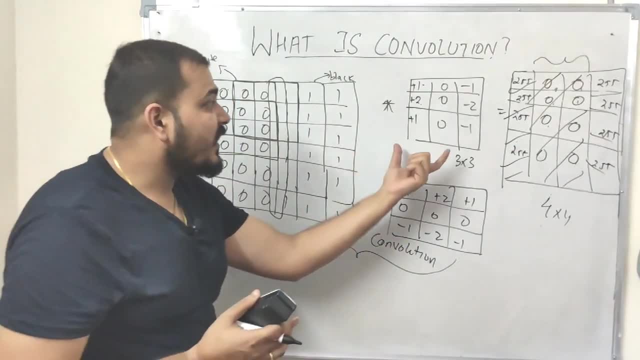 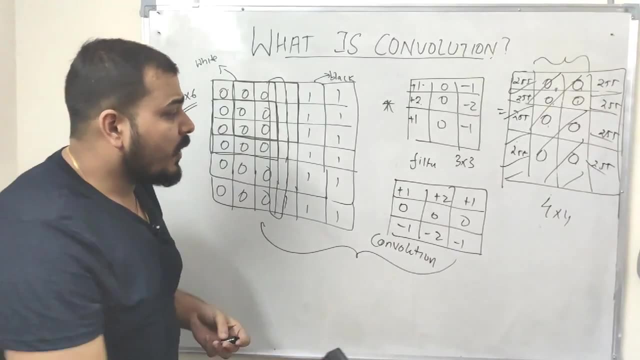 that we'll be discussing how we can do it, but just understand that this filter will play a very important role and we can consider any number of filters based on our image size and the problem statement. I also want to introduce you to one more formula. 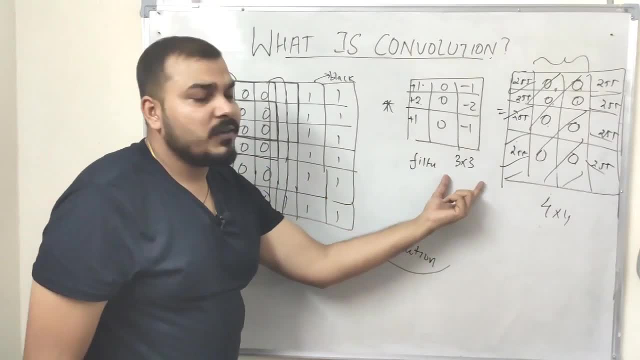 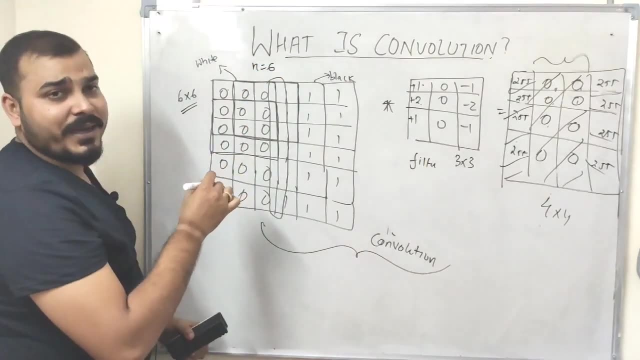 Now you see that I had six cross six image. When I applied a three cross three filter, I got an output of four cross four. So let me consider this: six cross six. I'm saying that the image size is: N is equal to six pixel. 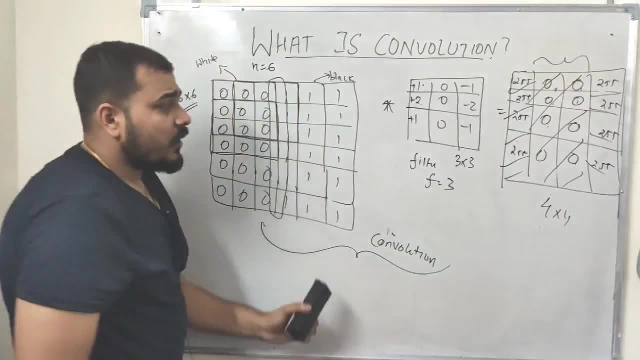 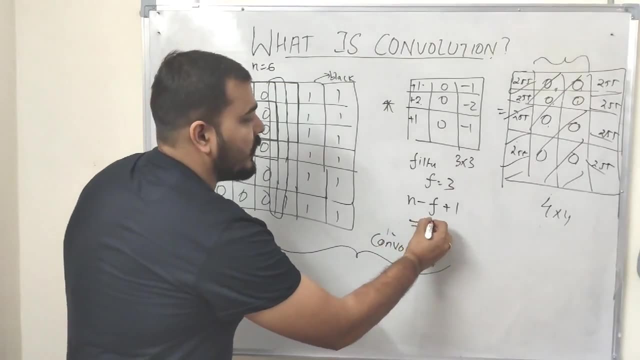 My filter size F is equal to three, My output is four. So for this we can basically apply a formula which is like: N minus F plus one. N value is basically my six value. My filter is basically minus three plus one. See, by applying this formula, 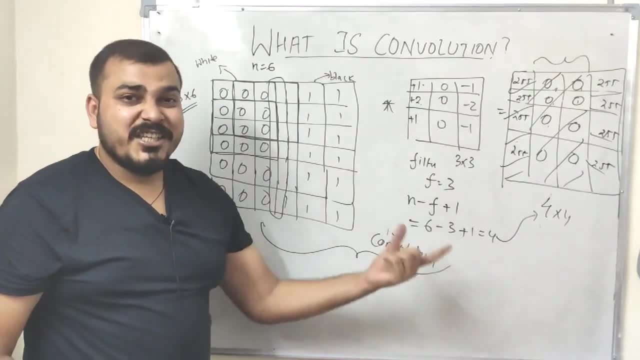 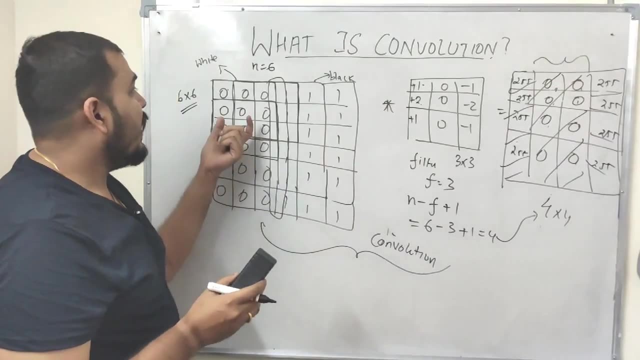 I'm getting the output as four cross four, but this formula will be changing, which I'm going to explain you in my next video, which is something about padding and stride. over here, I told you that stride is just one jump. Now suppose if we do two jumps? 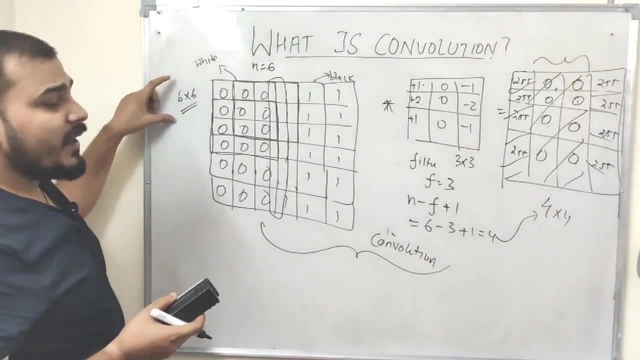 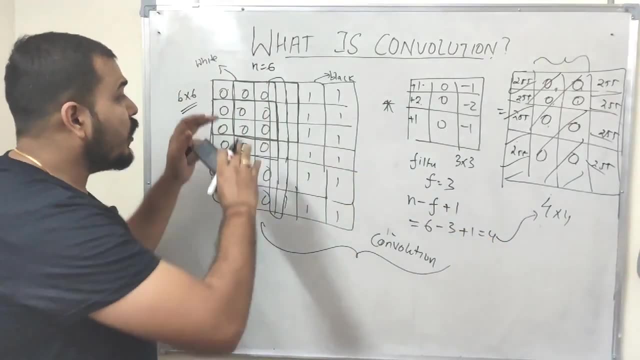 what will happen, And I'll also say you that if over here you could observe one thing is that the image size was six cross six, but now you're getting an image size of four cross four. That basically means you're losing some information from this image. 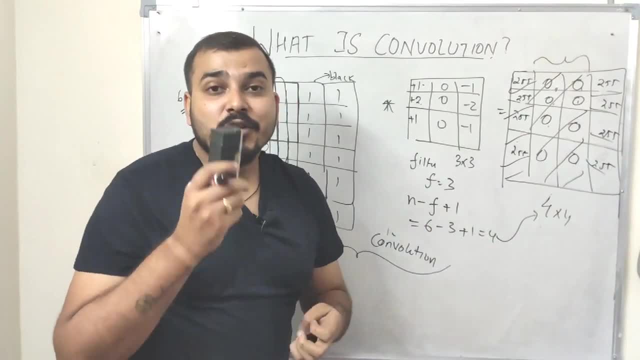 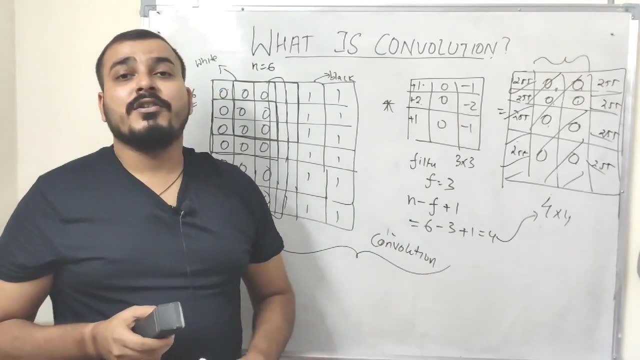 What if I want the same image size over here? So then you'll be implementing a concept called as padding and that will be discussed in the next video, and I'll also be continuing that- how that particular formula will also change. I hope you like this particular video.